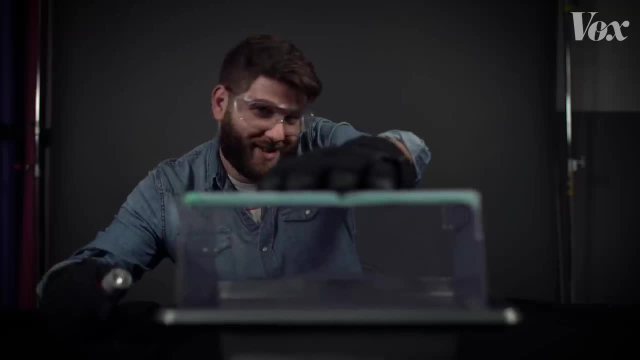 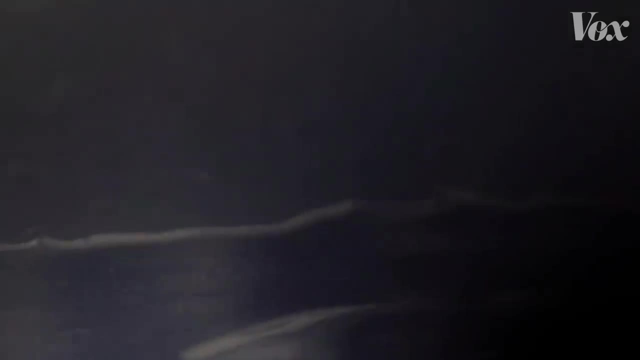 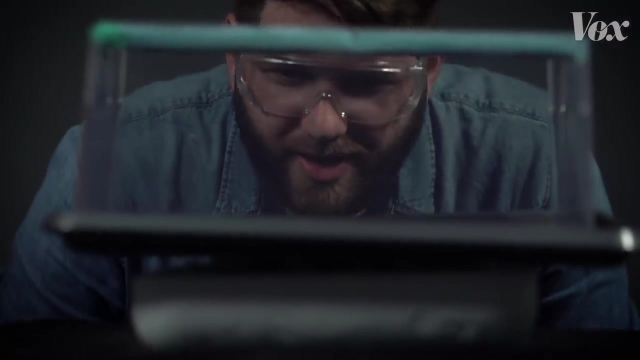 little droplets and you can actually trace their path through the cloud, Hopefully. Oh wait, wait, I saw one. Yeah, The particles in our cloud chamber are traveling from space at nearly the speed of light, as are the untold others passing by. 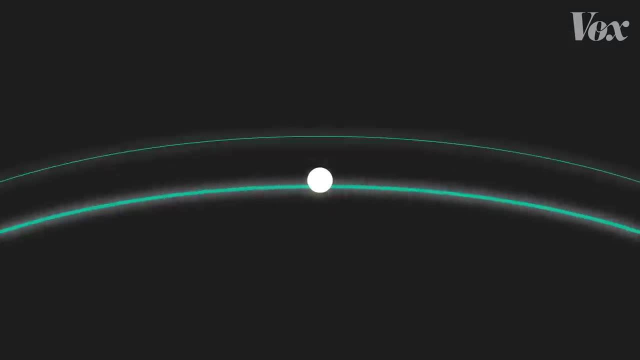 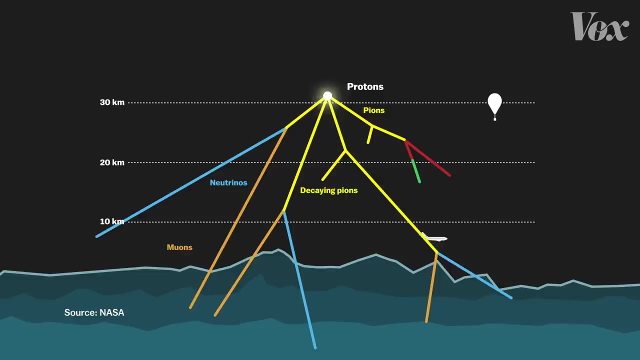 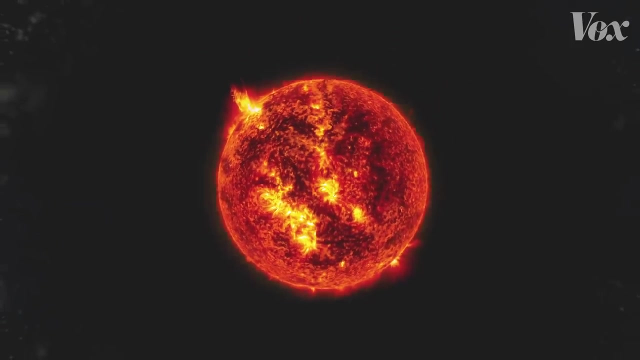 When they hit the top of our atmosphere, the impact is so powerful that the atoms of radiation burst open, tearing apart in violent cascading collisions. That's what we see in the cloud chamber: atomic shrapnel that has reached the ground. Scientists have determined that some of these rays come from the sun's atmosphere and the 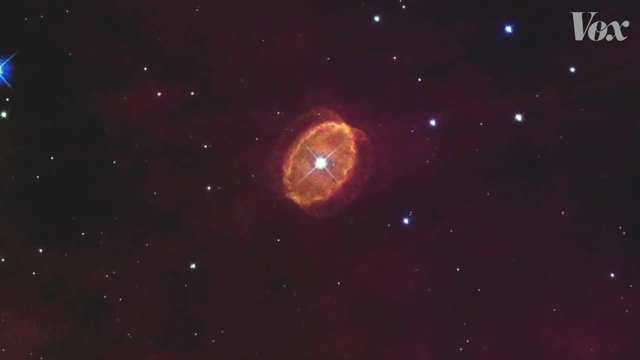 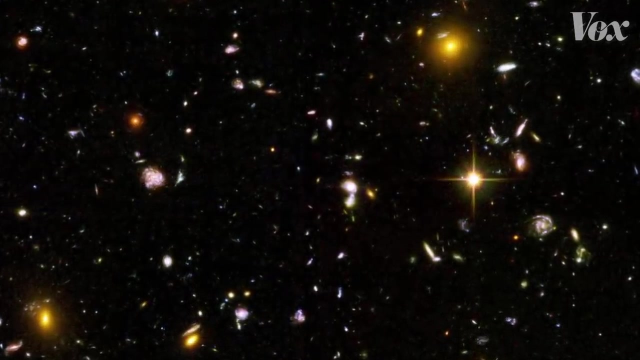 former solar wind and others from exploding stars. But the most powerful rays are the most puzzling. They don't even come from our own galaxy. They come from some unknown source out in the universe. The energy from the very most powerful ray recorded had enough power to turn on a light. 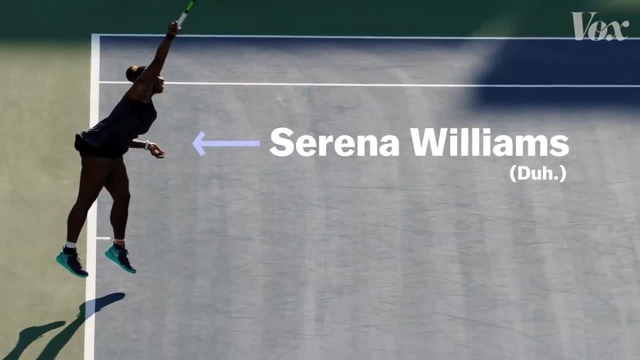 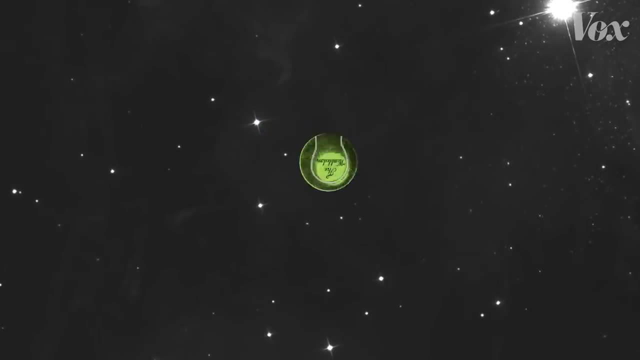 bulb for a second or more. That force is comparable to a top tennis pro hitting a ball with all their strength. Doesn't sound that impressive. but think of this: All of that energy is squeezed into an area smaller than an atom To try to figure out what entity could be shooting these incredibly. 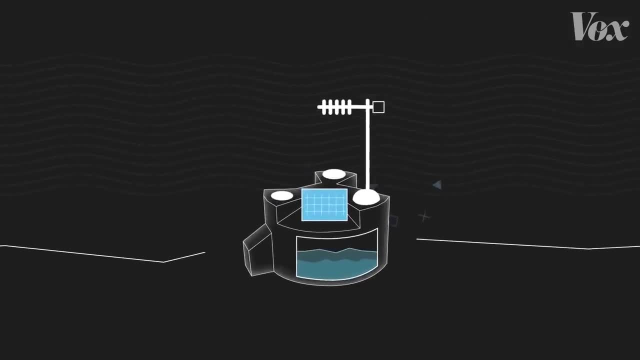 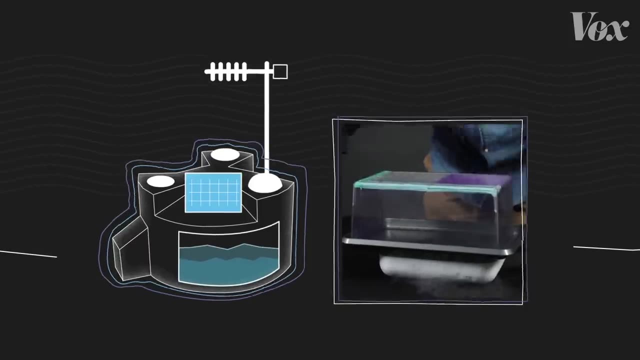 powerful rays at us. scientists used massive cosmic ray observatories with detectors not too different from our cloud chamber. Well, you know, that's a good thing: They're on a higher budget and they're more advanced. One in the South Pole uses a gigantic block of ice- a whole cubic kilometer. 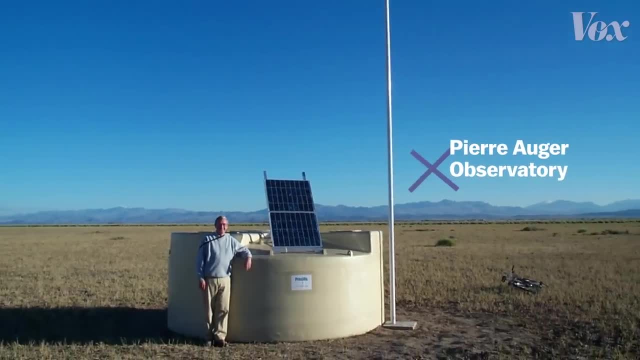 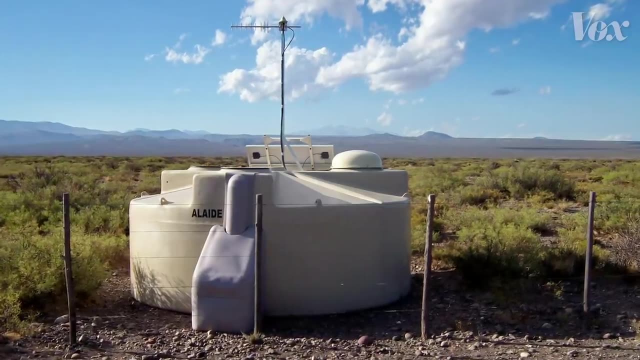 to track the rays instead of vapor. Another one in Argentina has 1,600 huge water tanks spread out over 1,000 square miles. But instead of just observing cosmic rays as they shoot by, scientists used sophisticated technology to trace the atomic shrapnel backwards. 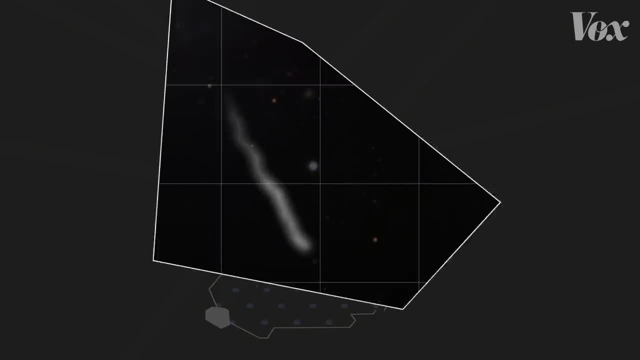 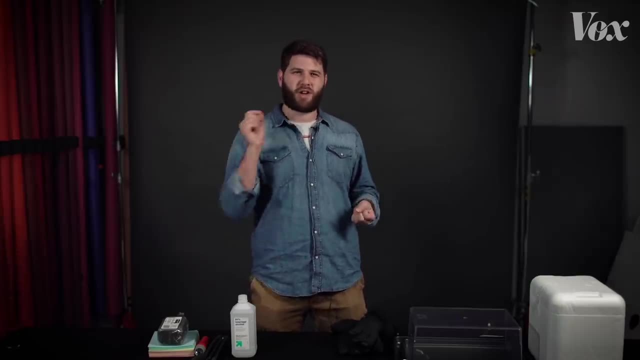 There they can reconstruct the original cosmic ray that hit the top of the atmosphere. But confirming their source in the deep reaches of space isn't so easy, because these cosmic rays don't always travel in a straight line. Instead, the various magnetic fields of the universe and the galaxy 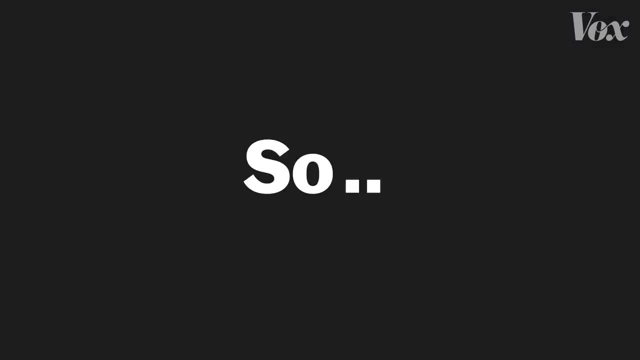 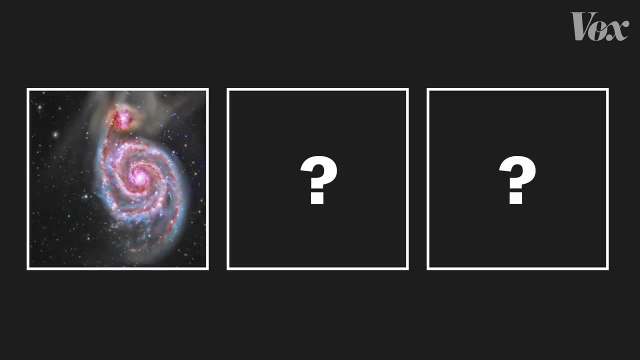 put them on bendy paths. So are there any ideas where they come from? Scientists have a few suggestions. The cosmic rays could be created in the violent hearts of galaxies far away. Another leading hypothesis is that they're not produced by exploding stars per se.